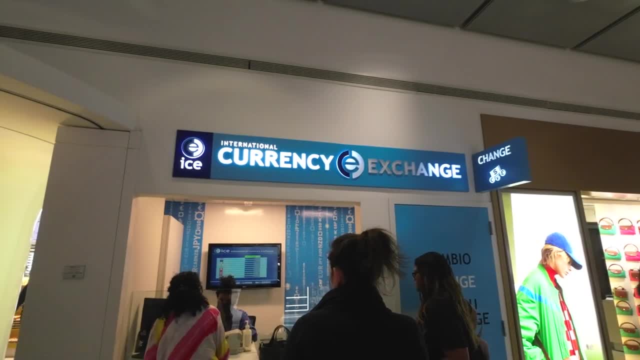 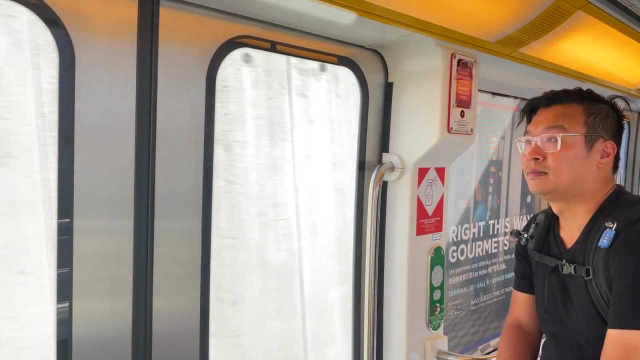 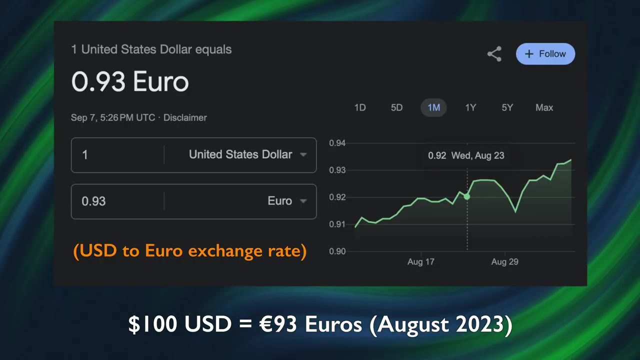 for exchanging currency. From my experience, you're losing close to 40 percent in the exchange process. here I'm going to be using a few real life situations. The examples I'll be using are timed during August of 2023.. In the next clip I asked one of the vendors at an airport exchange. 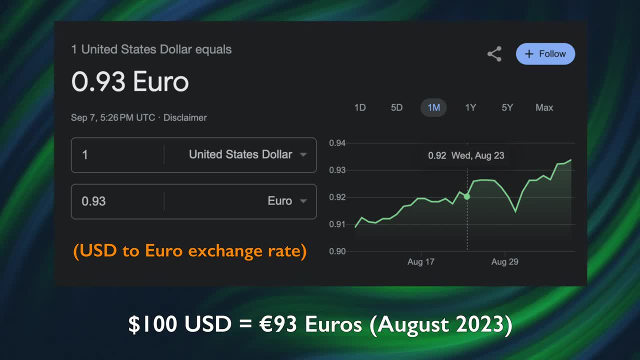 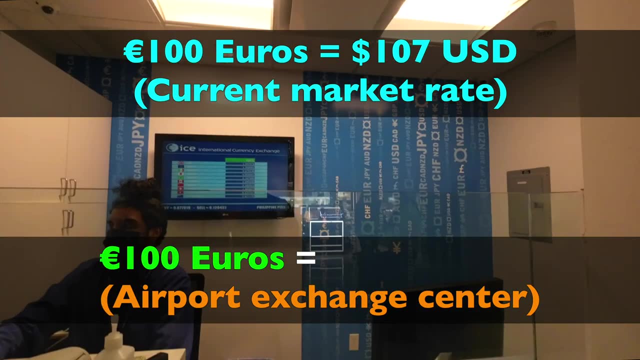 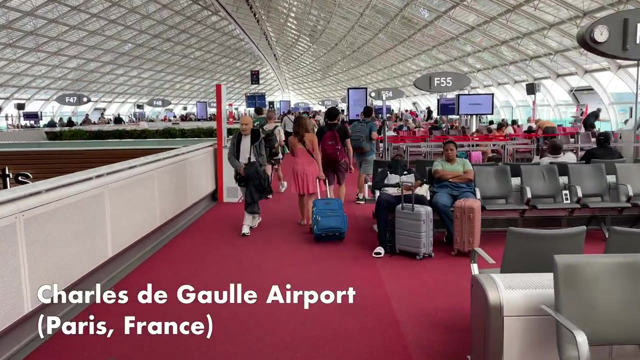 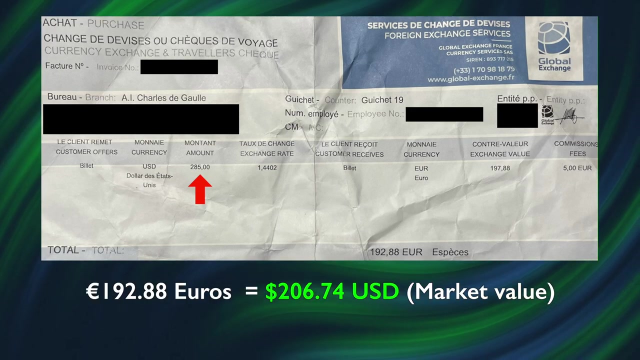 center on what the exchange rate would be for 100 euros and US dollars. Let's take a listen. What about 100 euros? 148?. I ended up having to use one of these exchange centers only because I was not sure if I had enough euros with me during my trip to France. So for 192.88 euros. 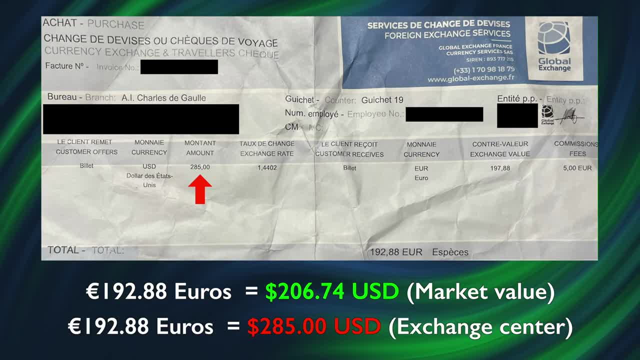 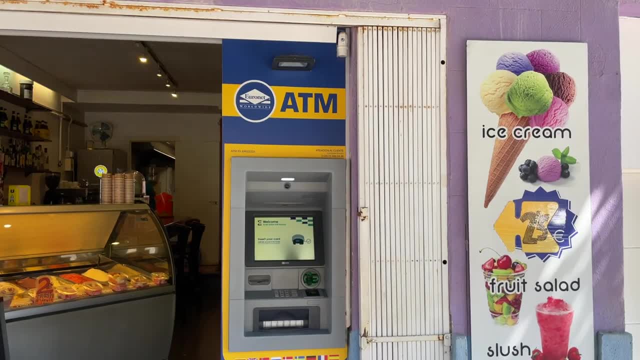 I ended up having to shell out 285 dollars. I was close to losing roughly about 40 percent on this one currency exchange alone. The next clip I'm going to show you is the most common way to get a fair exchange rate without using these ATMs. The next one up on this list is ATMs, and specifically a company called. 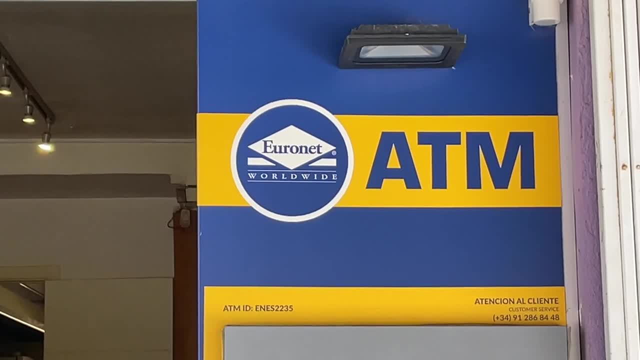 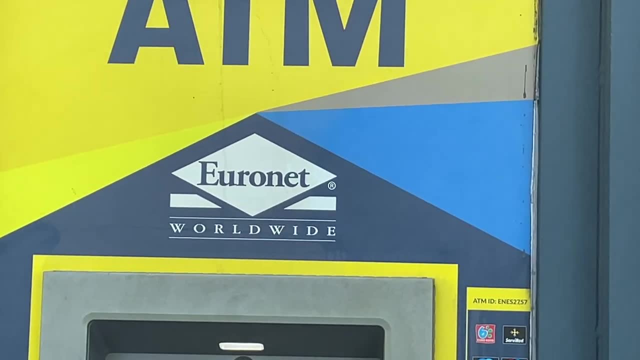 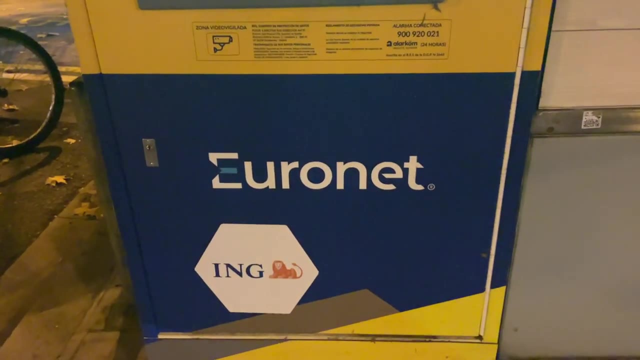 Euronet, which is found in most European countries. You are losing roughly about 20 to 30 percent when using these ATMs to exchange currency. What's worse is that some of the touch options on these ATMs are in very large amounts and sometimes can go as high as the entire salary for a typical. 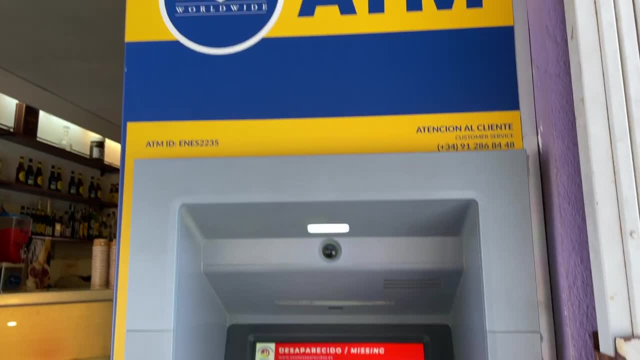 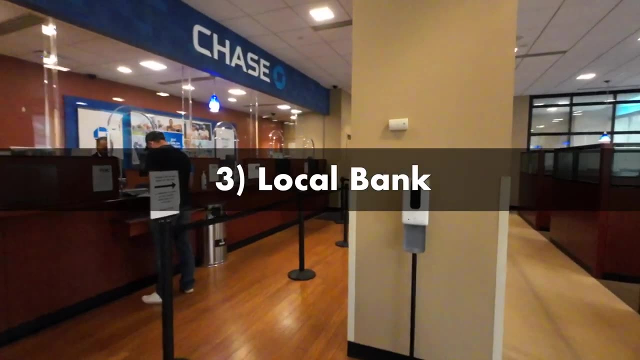 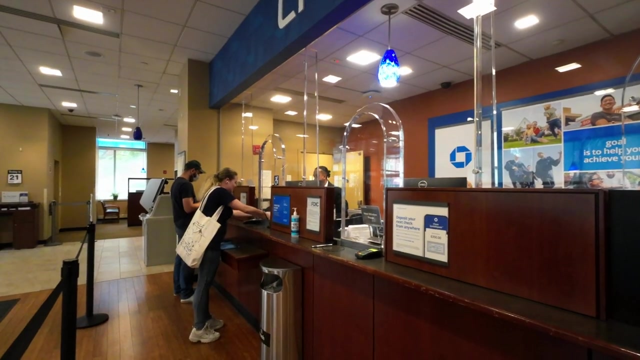 European. It's also not even a European based company. It's an American company. so go figure. The last option for exchanging currency, which happens to be the best option, is your local bank. You're still losing about five or six percent in bank fees, but it is the best option out of. 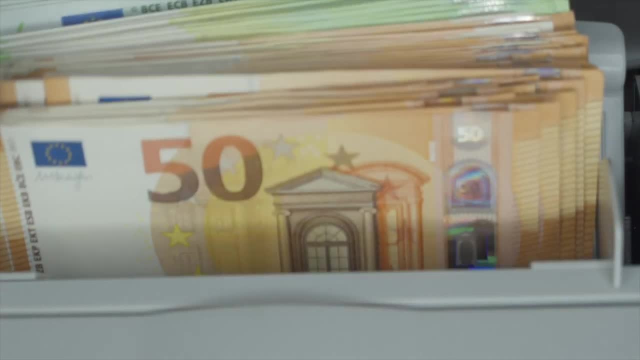 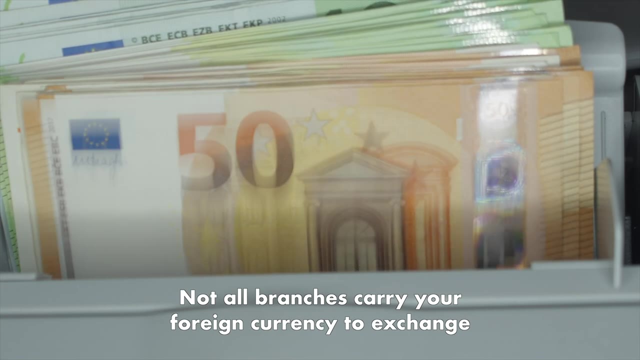 what is available to you. You will need to check which branches currently carries your foreign currency. Not all of them have them in stock. I use Chase Bank, for example, and in Brooklyn they had about five branches that carried euros. If this is not appealing to you, you may have to ask your. 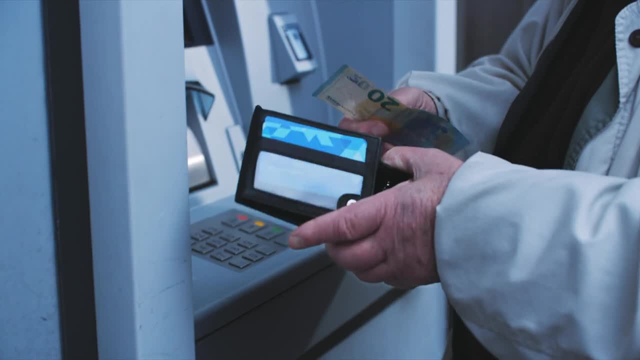 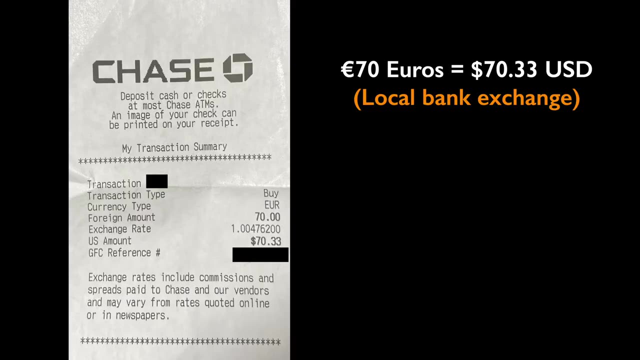 bank to order your foreign currency for you. I had some leftover euros from my trip and in this situation you can just bring it back to your local bank to exchange it for US dollars. This is my receipt and I had about 70 euros to exchange. The exchange rate was close to a one-to-one ratio. which means that I was losing about seven percent on this transaction, which is not terrible compared to your other options. Just keep in mind that in most major cities they do take credit card, so you may not need as much cash as you think. If you do decide to use a credit card, just make sure that that card has no foreign transaction. fees. So you're looking to use travel cards such as the Chase Sapphire Reserve or the American Express Platinum card to use in this situation. Otherwise, you would incur a three percent foreign transaction fee on every purchase. So there you have it. Going to your local bank offers the best.